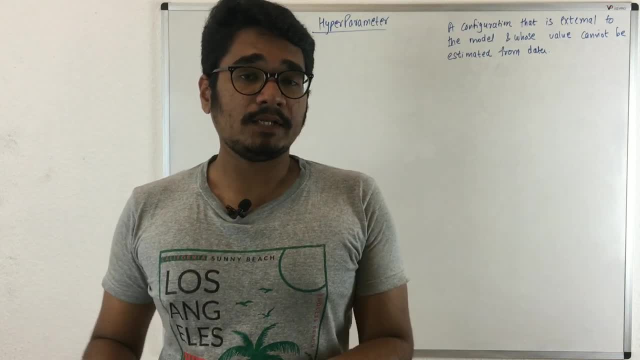 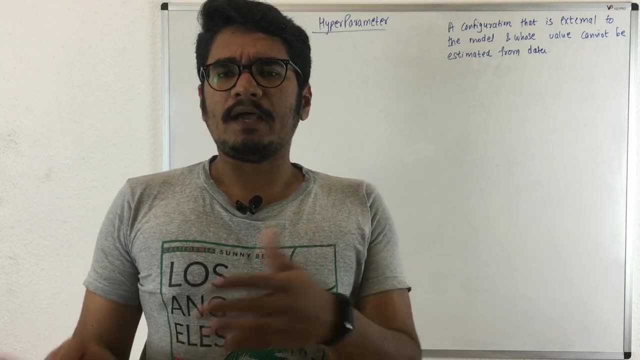 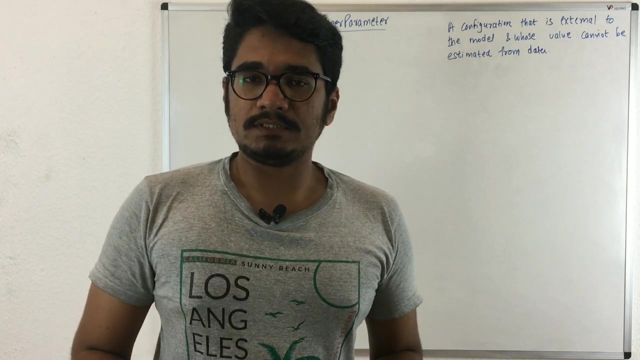 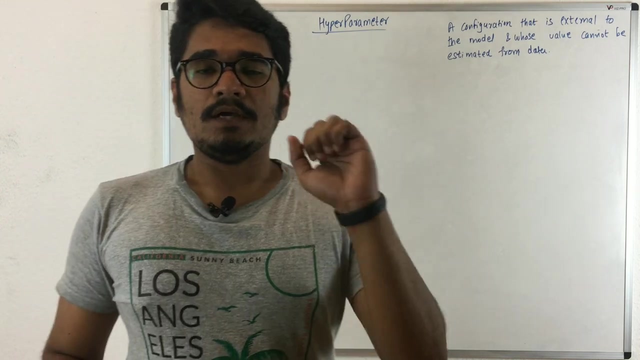 Welcome back to my channel. So far we have seen different types of classifier evaluation methods in machine learning. That is, we saw the holdout method, We saw the random subsampling and then we have something called as cross validation and nested cross validation, in order to overcome the limitation which was there by the random subsampling. So before that, I thought the need of explaining a concept called as the hyper parameter. Why? Because this term or this concept is mainly used in cross validation as well as nested cross validation. 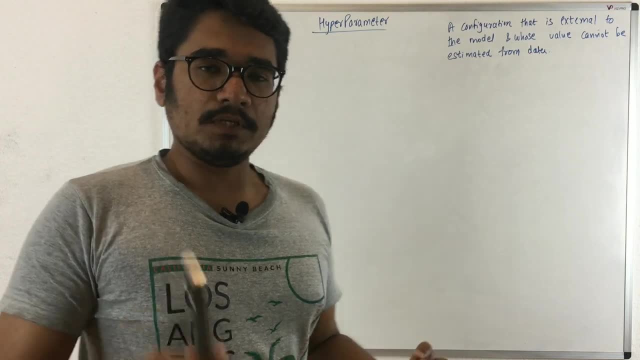 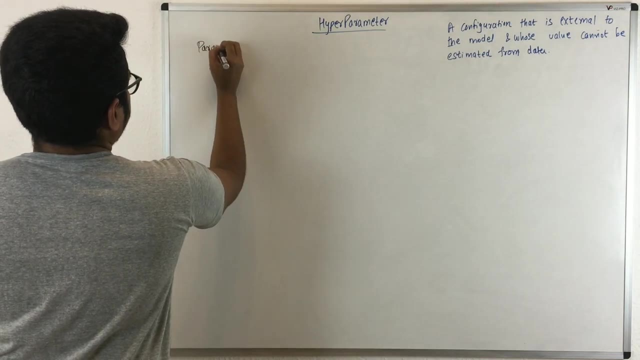 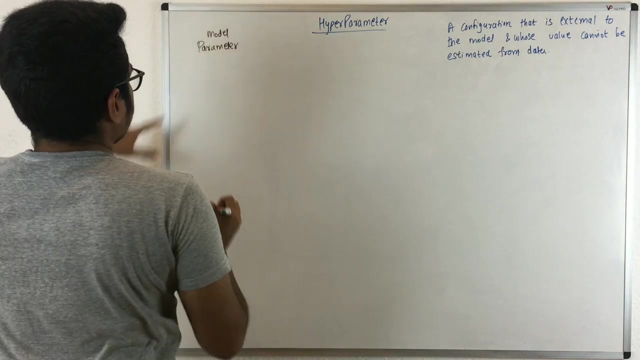 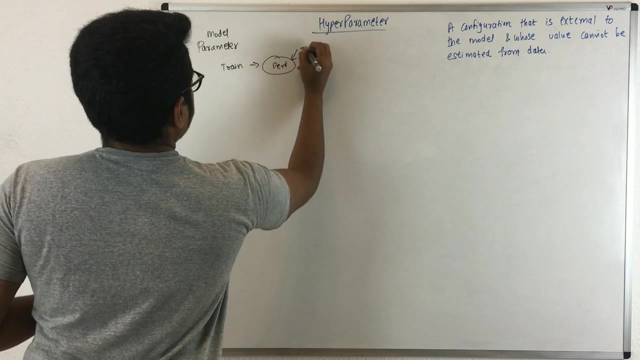 So in today's video, let's see what is hyper parameter, So let's begin. So, basically, before starting with the hyper parameter, let us consider the term that is parameter. Now, since we are learning about the machine, we have created a model. So the model you get from your training data and then you evaluate its performance based upon the test data. So here what you have is basically in: 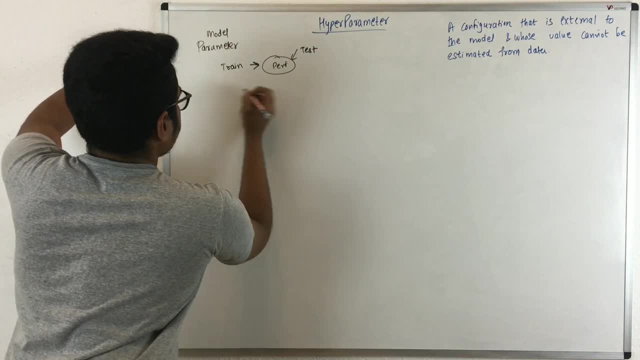 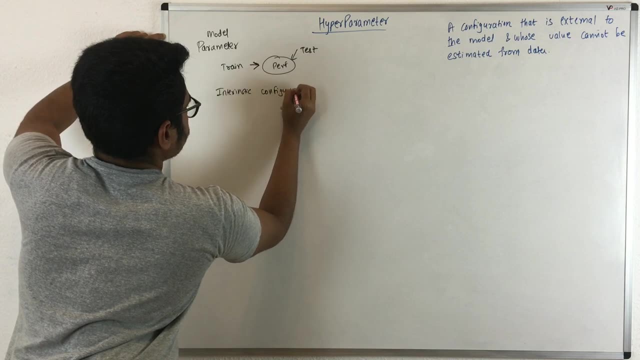 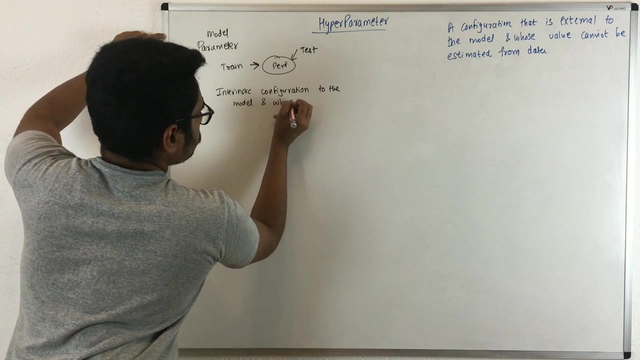 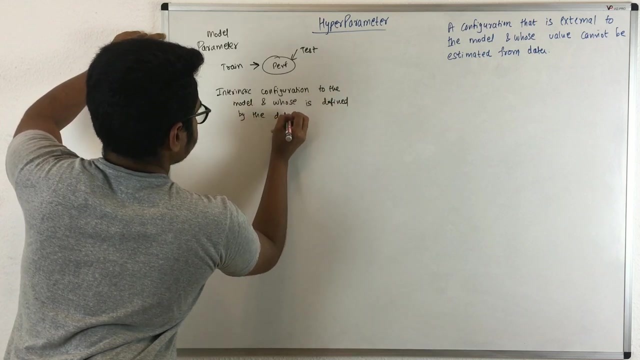 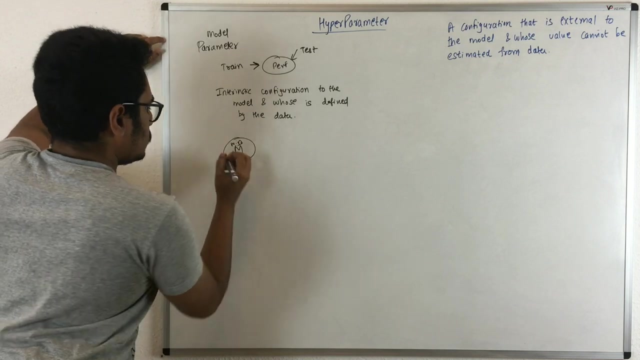 machine learning. that is the model parameter which is there, that is an intrinsic configuration to the model and whose value is defined by the data. Now what this basically means is say you have a model- Now this could be naive bias- and say, for example, it has three parameters: p1, p2, p3 and what it? 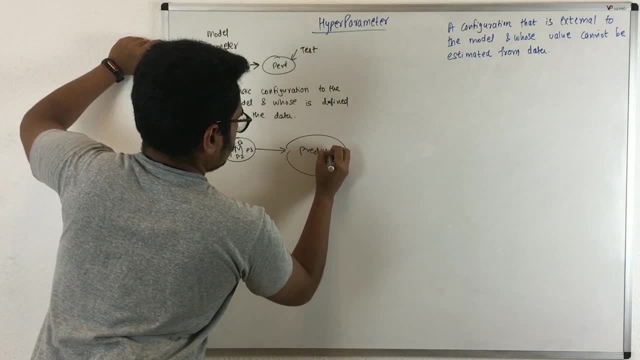 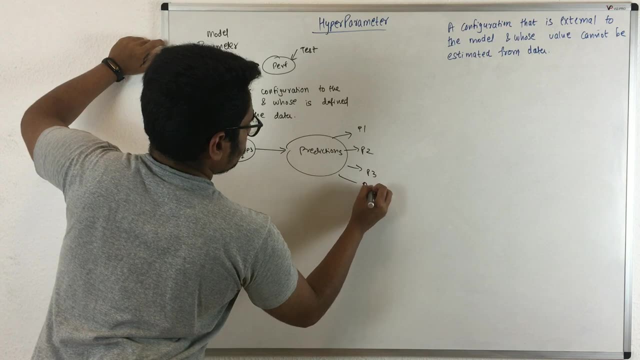 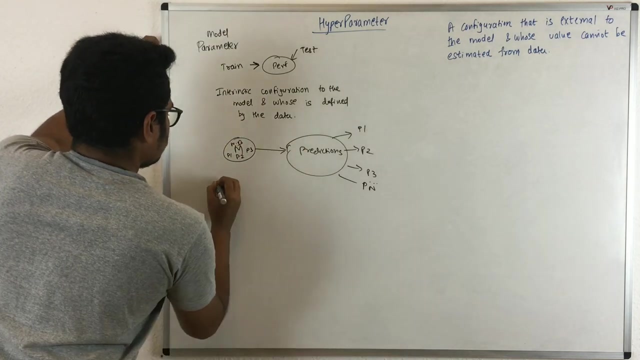 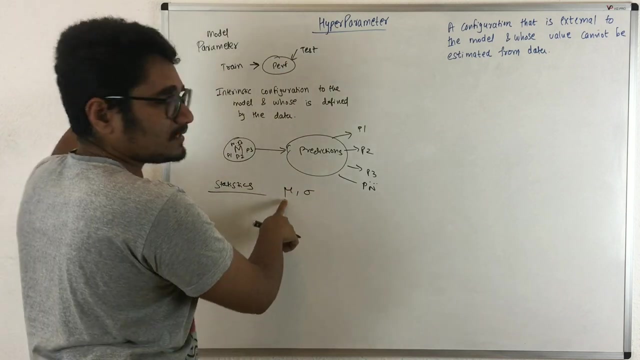 does is it does the predictions. So predictions could be prediction 1, prediction 2, prediction 3, or you have prediction n, so it creates n number of predictions based upon the values it gets. So in terms of statistics we have, say, mu and sigma parameters. So mu is the mean and Sigma is a standard deviation. 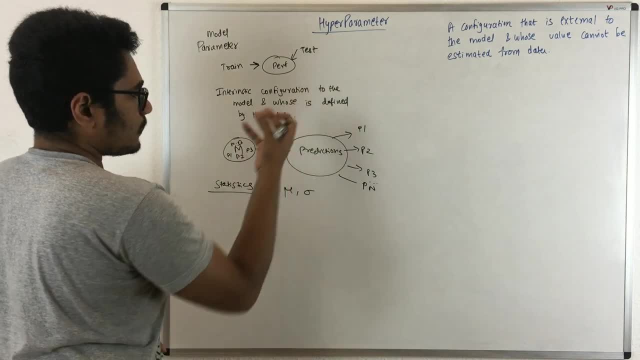 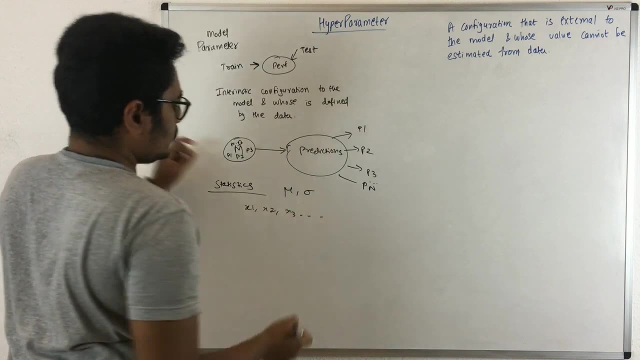 So if you want to derive these parameters, we derived from the data that we have. so we have some data points or a stream of data- X, 1, X, 2, X, 3- and based upon that you derive this, and if you want to estimate the normal distribution, then we use this parameter that. 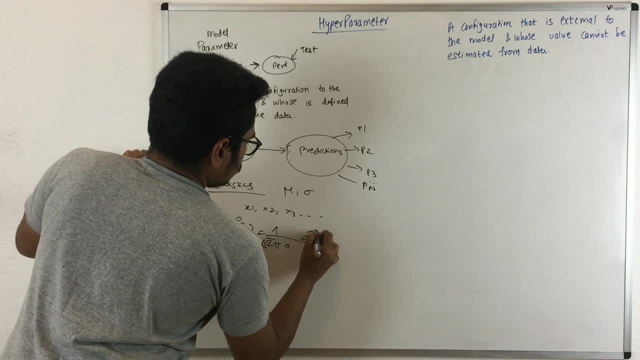 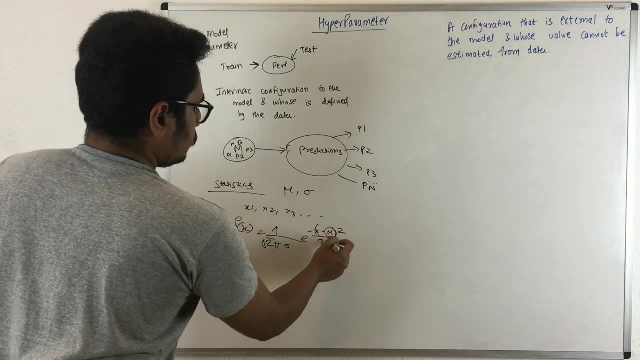 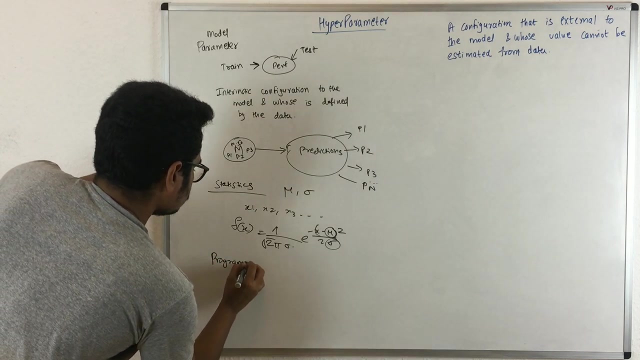 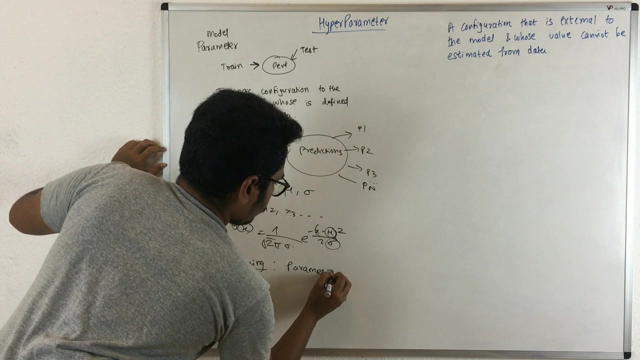 is in this formula, E raised to X minus mu, the whole square upon 2 Sigma. So with this is you just put the value of mu and Sigma into this and then you estimate the function. for this in terms of programming, You have a concept called as parameterized method. 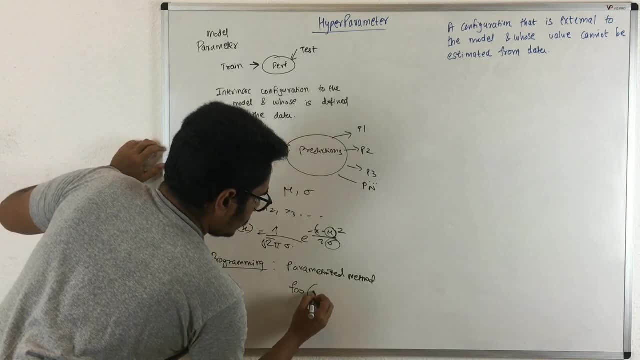 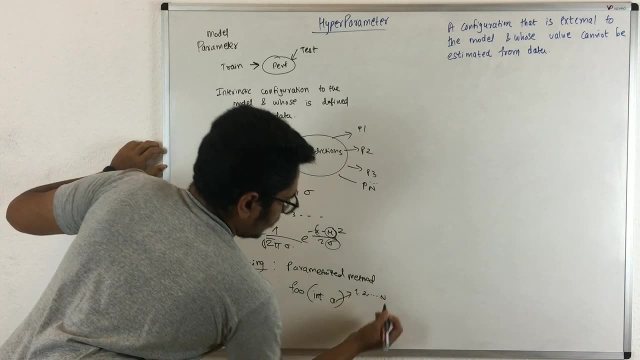 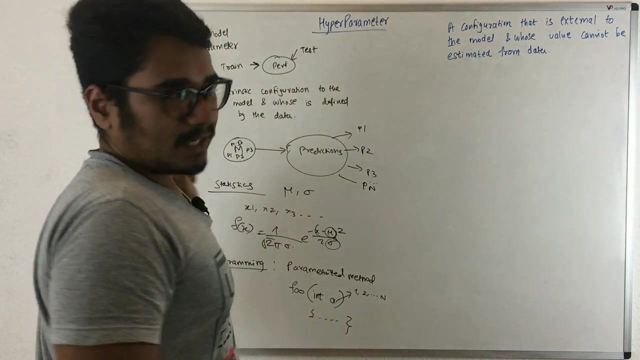 So say, for example, you have a method foo and it has got a parameter that is int, a means. it takes all the integer values, So it can take any values up till n, and it has further lines of code defined by the programmer. Now this is the basics of the model parameter. 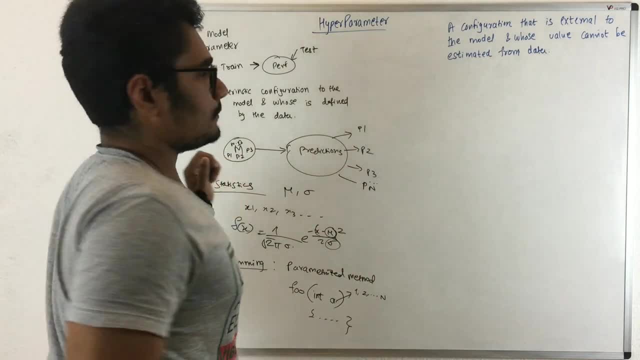 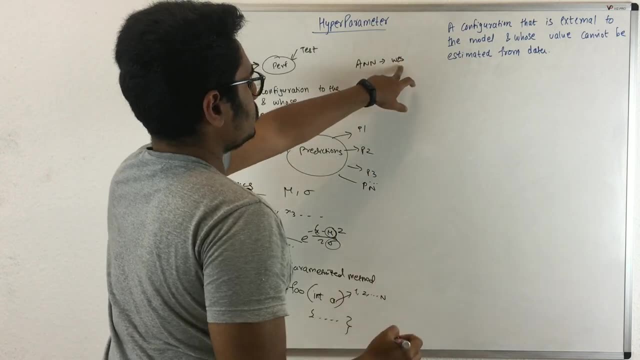 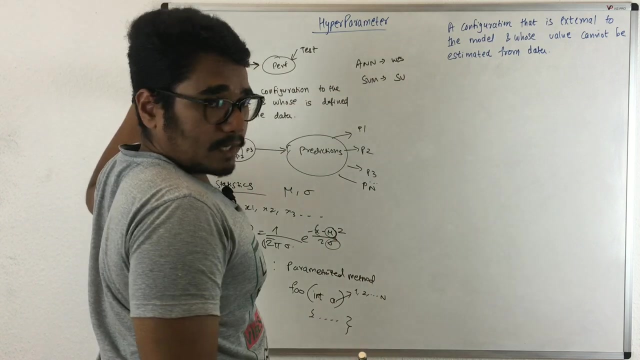 which you already know. now in machine learning, where this concepts are used, So in artificial neural networks, we have something called as weights which are associated with this model. So this weights are nothing but the model parameter. in support vector machine You have the support vectors which are model parameter. or in support vector machine you 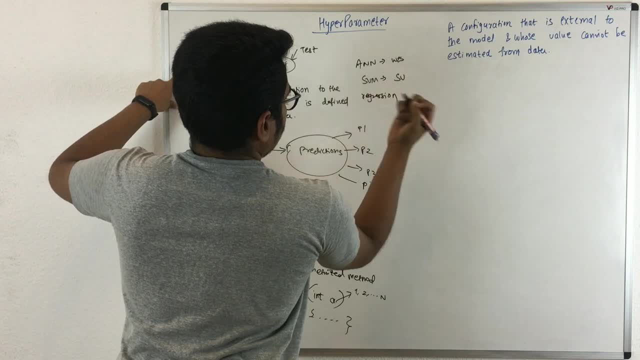 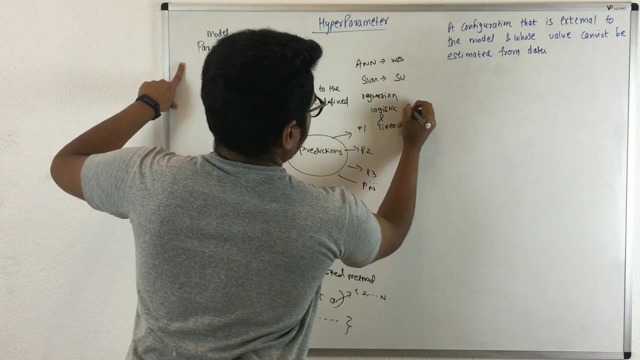 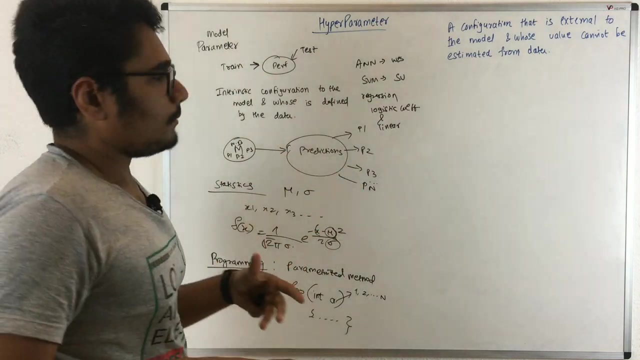 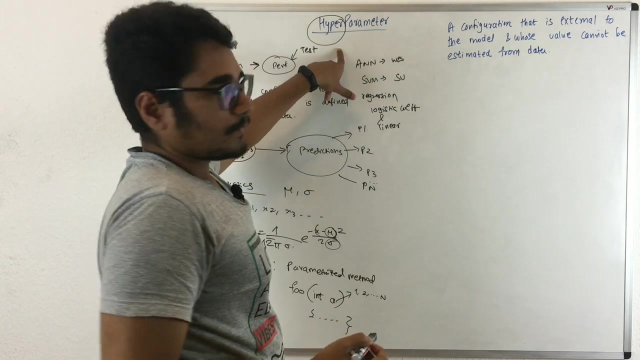 can regression. Specifically, when you deal with that is, logistic and linear regression, you have some coefficients, So this coefficients are nothing but the model parameter. Now, this was all regarding the model parameter. now let's deal with the term hyper parameter. so it has got one prefix Before the term parameter, so let's go with the definition. 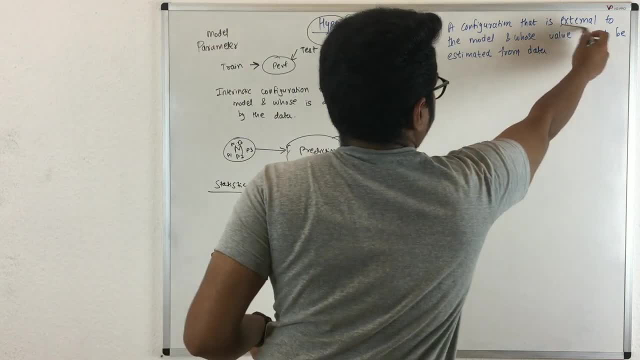 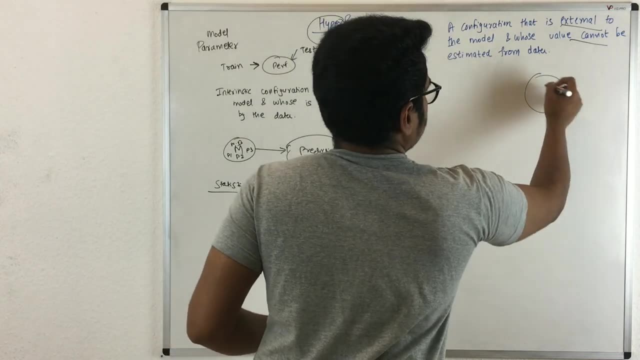 So it's a configuration that is external to the model. So it can be defined as classes. so it's a configuration that is external to the model model and whose value cannot be estimated from the data means, whatever you give the hyper parameter. So consider, say this is a model and you just provide this externally. 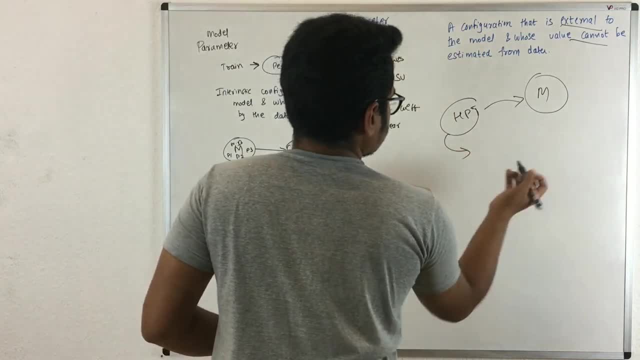 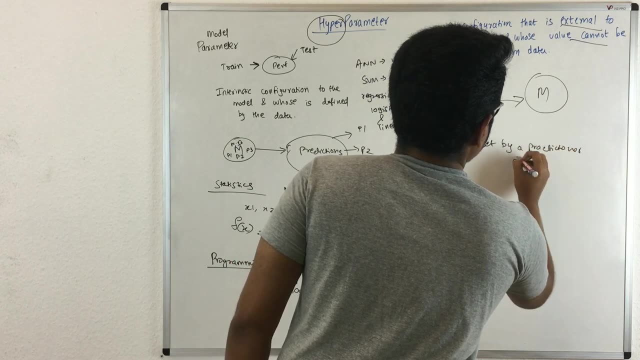 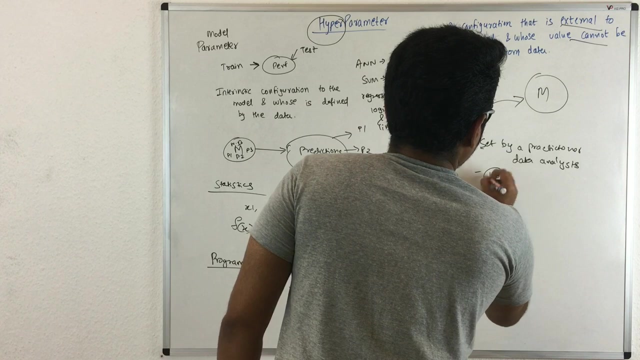 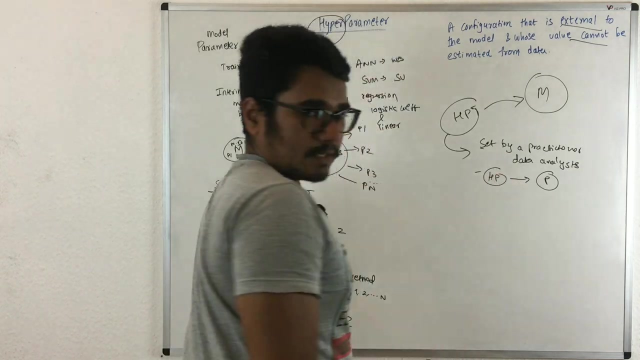 Now hyper parameter has got three things to deal with. So first, it is set by a practitioner, So practitioner could be your data analyst. Second is hyper parameter is used to derive the model parameters, means before the model parameters are derived, you set the hyper parameter externally. and third, is hyper parameters derived. 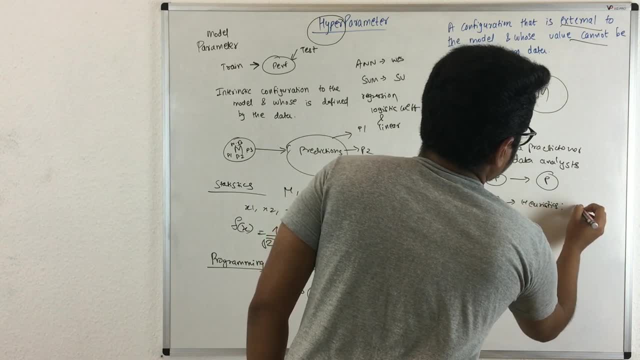 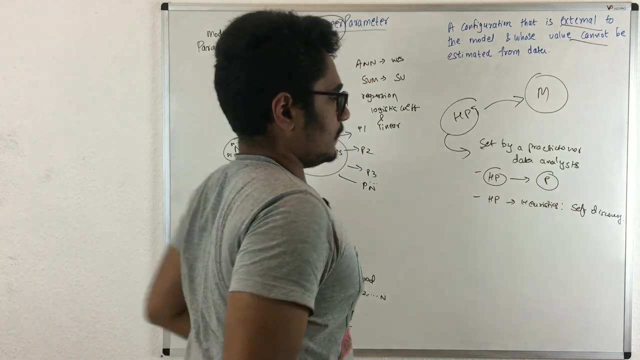 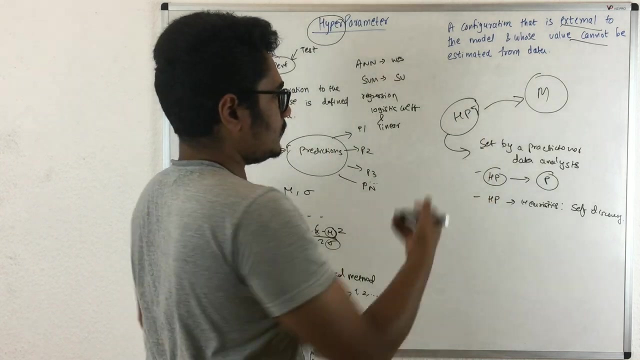 from heuristics Means there is a self-discovery of the value instead of its being automatically set. Now, these are the three things which are associated with the hyper parameter. Now, where in Machine learning, hyper parameter is used, say, we have already seen the KNN model. 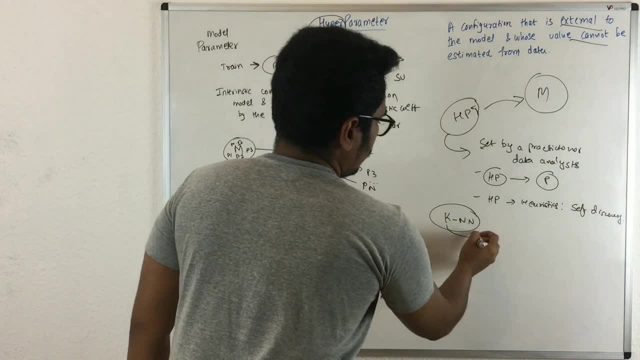 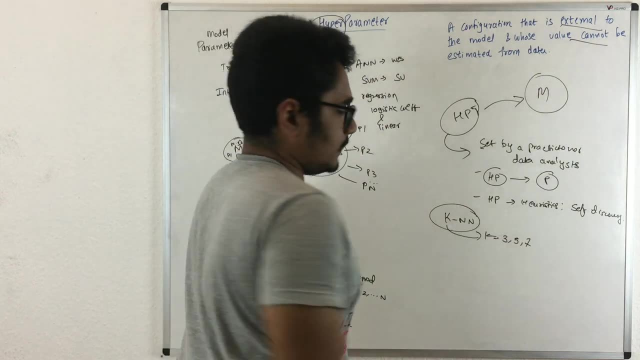 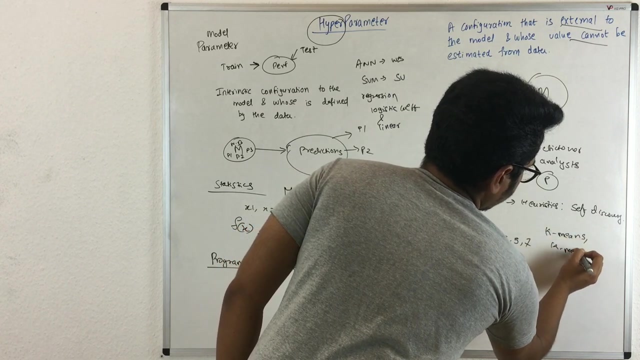 So that is the K nearest neighbors and we define the value of K, that is, K is equal to 3, 5, 7. that determines the number of nearest neighbors which it has. or if you have the clustering algorithm, say K means and K Medoids, you have this parameter, that is, you need to. 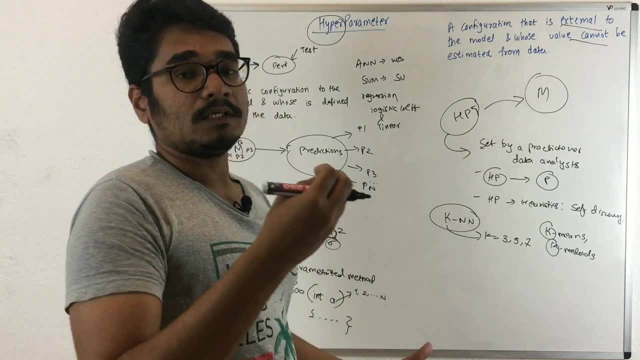 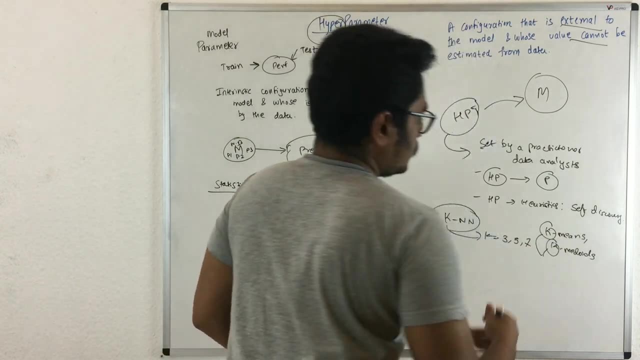 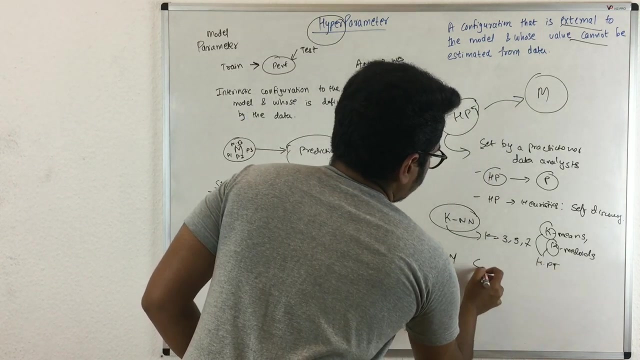 define the number of Cluster Clusters which you want to have, that is, if you want to have three clusters or five clusters, you need to determine it predefined. So this thing which you determine previously, before studying our algorithm, that this is nothing but the hyper parameter or in support vector machine, we have some terms or some. 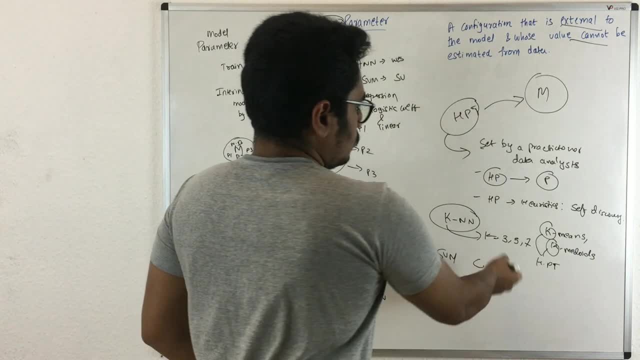 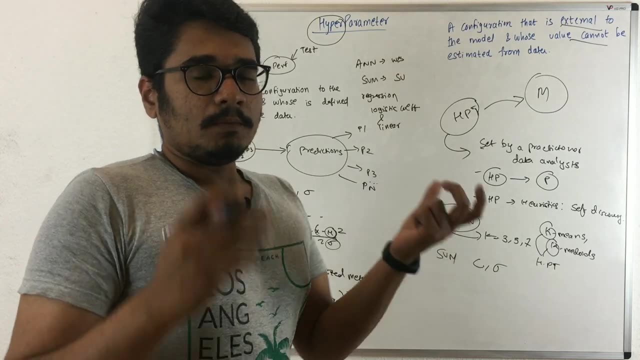 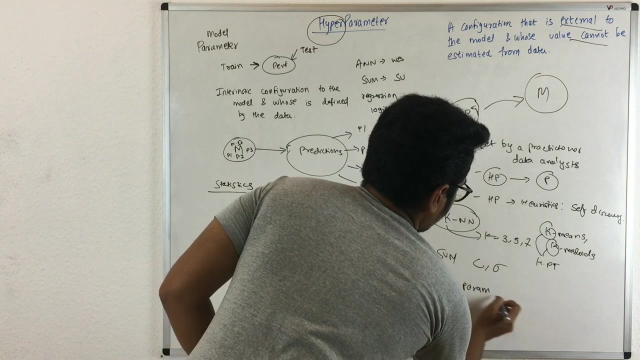 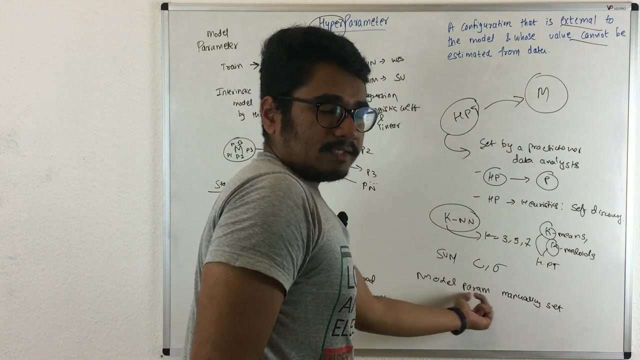 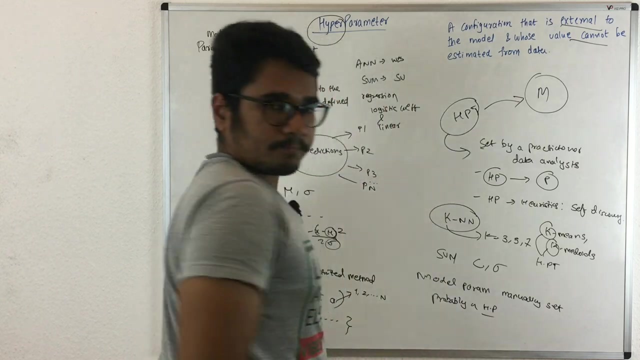 parameters like C and Sigma. So these are nothing but the hyper parameter which you set externally. Now how to differentiate between a model parameter and a hyper parameter? So if you have a model parameter And it is manually set, Then if this parameter is manually set, then this is probably a hyper parameter. 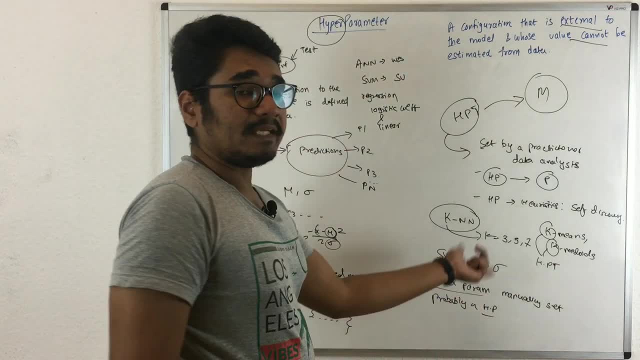 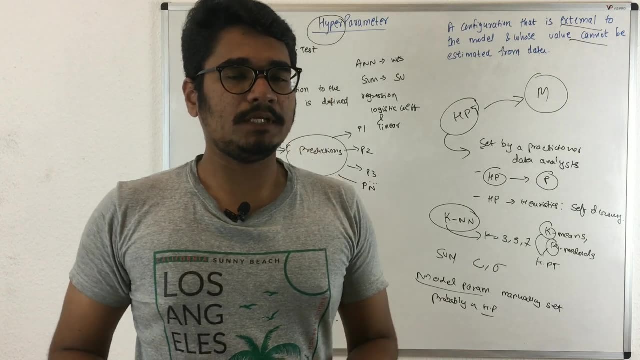 So if you don't manually set it, then that becomes a model parameter, But instead, if you set manually, then that becomes a hyper parameter. So well, That was all About the hyper parameter concept in machine learning. So hope you guys enjoyed this video and if you are watching this video, please do like. 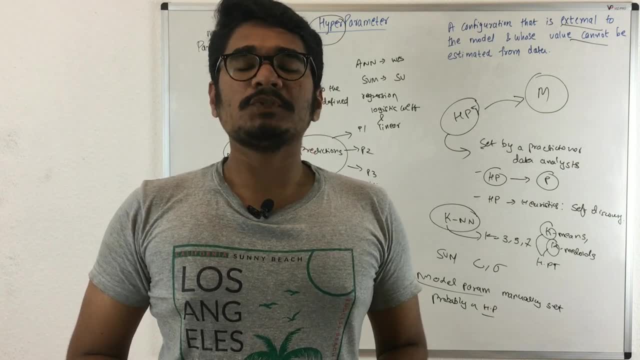 share comment and if you are new to this channel, please consider subscribing. Thank you very much for watching this video.